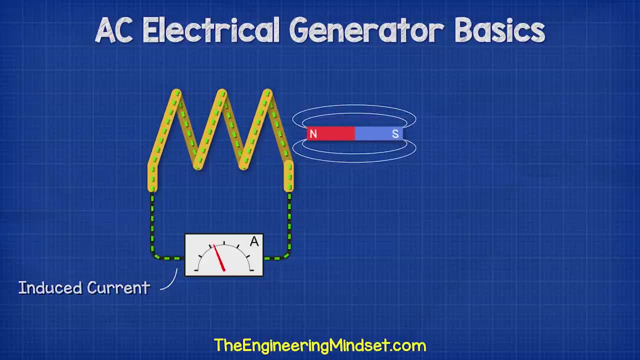 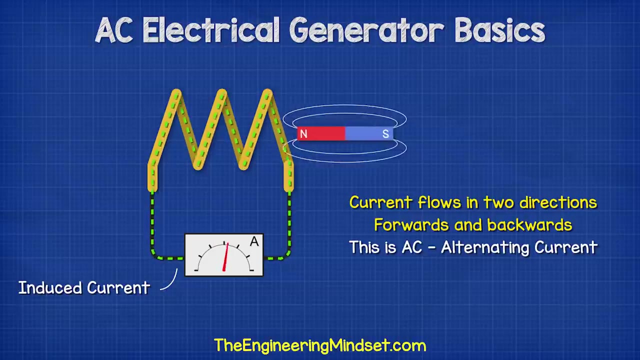 the current flows in the opposite way and the dial indicates a reverse current. If we move the magnet in and out repeatedly, the current will therefore alternate between flowing forwards and backwards. This is how AC, or alternating current, is generated. The current is continuously alternating in direction. 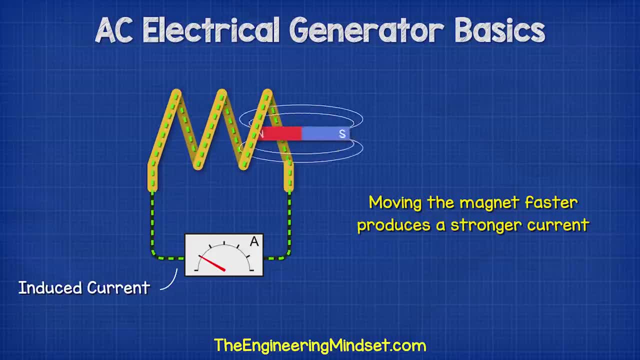 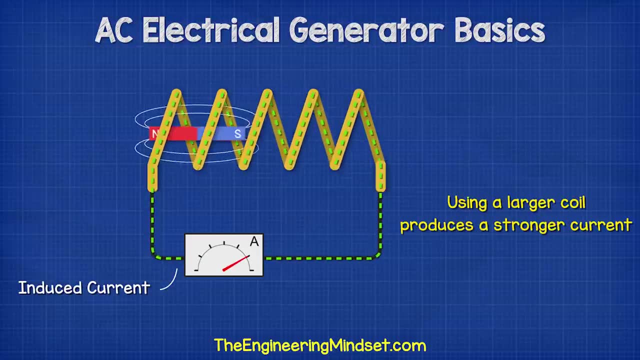 If we move the magnet faster, a stronger current is generated. If we use a stronger magnet, then the current also increases. If we use a larger coil with more turns, then this will also generate a larger current, Instead of using a permanent magnet. 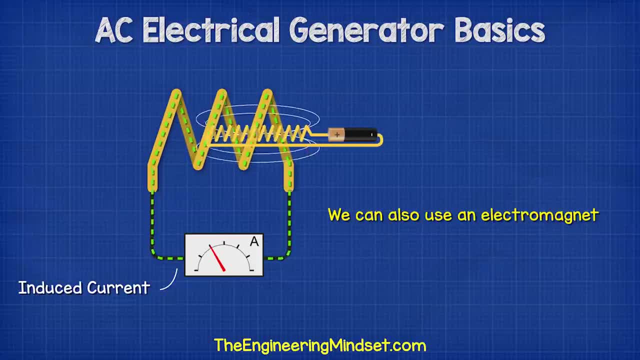 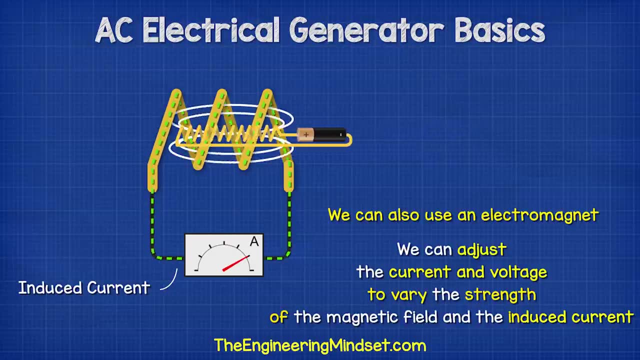 we could use an electromagnet. As we move this in and out it will also generate an AC current in the coil, But with the electromagnet we can adjust the current and voltage to vary the strength of the magnetic field. This lets us control. 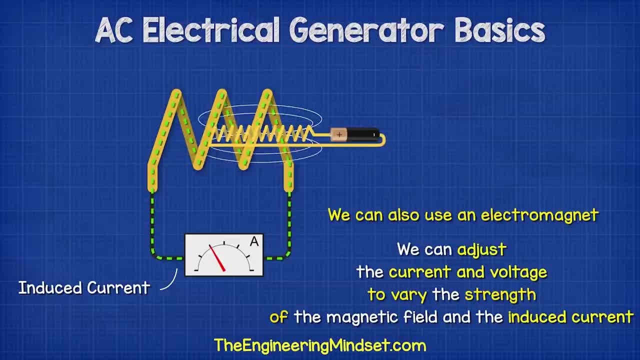 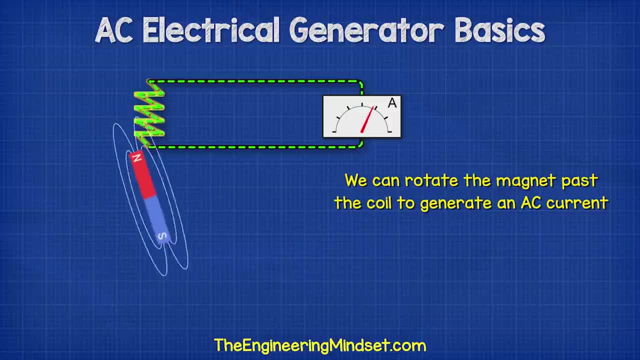 how much current is generated in the coil. Instead of moving a magnet in and out of a coil, we can generate a current much easier by rotating the magnet and placing the coils around this. The strongest part of the magnetic field is at the ends. 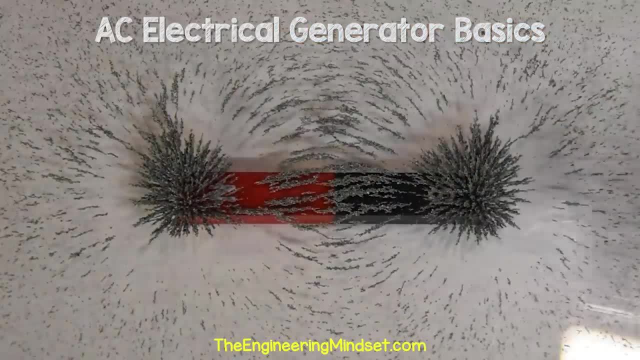 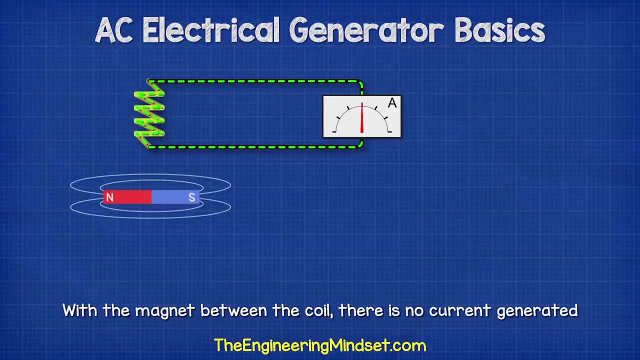 where the magnetic field lines converge. You can see the magnetic field lines by sprinkling iron filings over the magnet. With the magnet between the two coils there is no current generated, But as the magnet starts to rotate, the strongest part of the magnetic field. 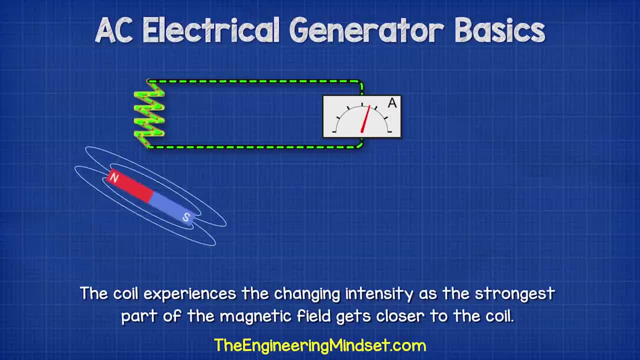 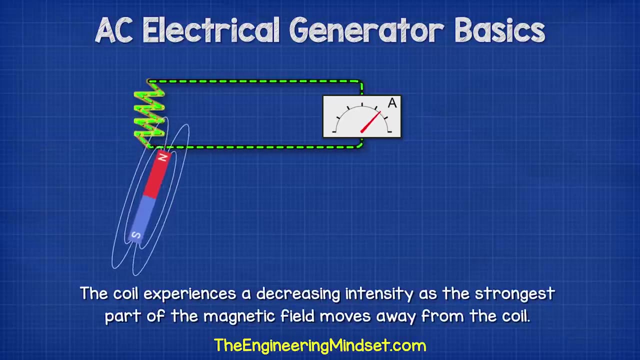 gets closer and closer to the coil, The coil experiences a changing intensity of the magnetic field. This will cause more and more electrons to be pushed forwards up until its maximum strength. Then the magnet starts to move away from the coil, So the magnetic field begins to decrease. 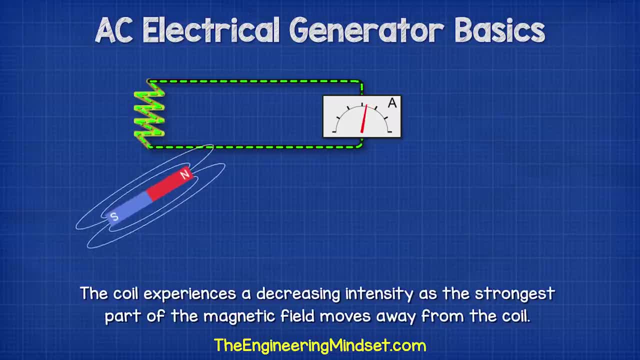 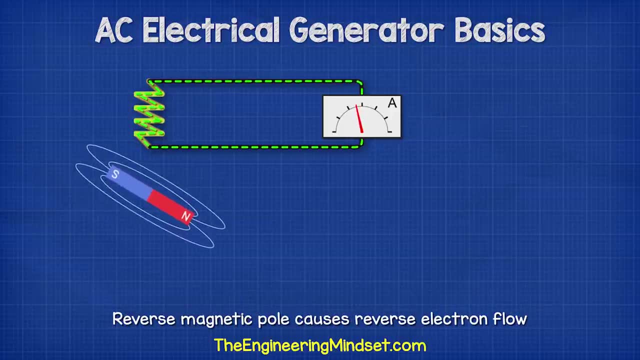 and so does the current of electrons, until it reaches zero again. And now the opposite end of the magnet begins to get closer to the coil, and this pulls the electrons in the opposite direction. This again reaches a maximum point and then decreases back to zero. 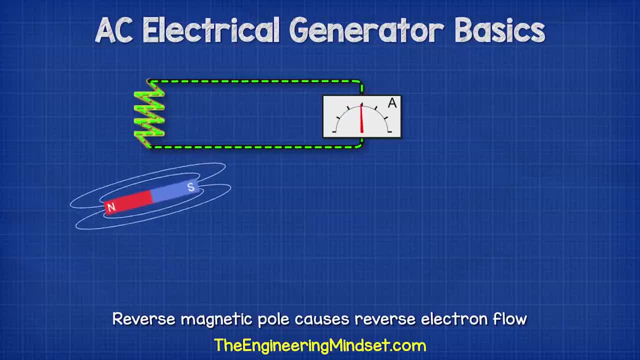 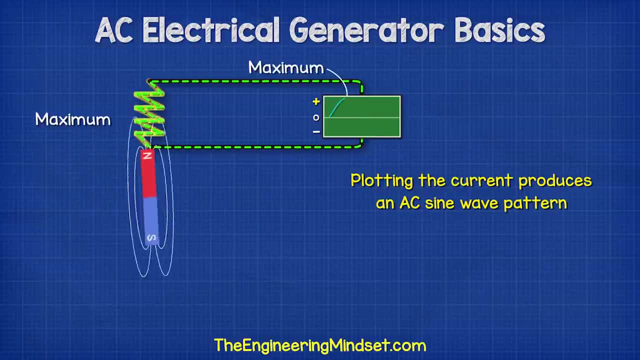 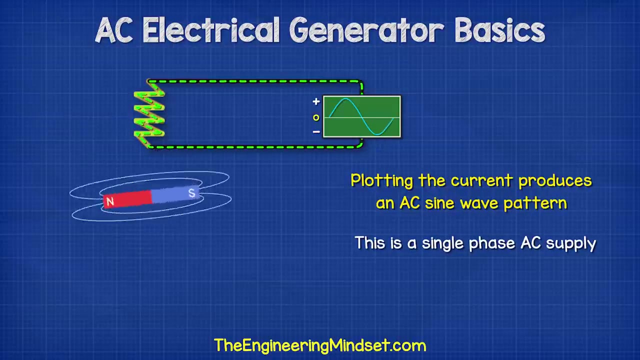 And so if we were to plot this current on a chart, we would get the current in the opposite direction. We would get a sine wave, with a current flowing in the positive and then the negative regions. This setup gives us a single phase AC supply.